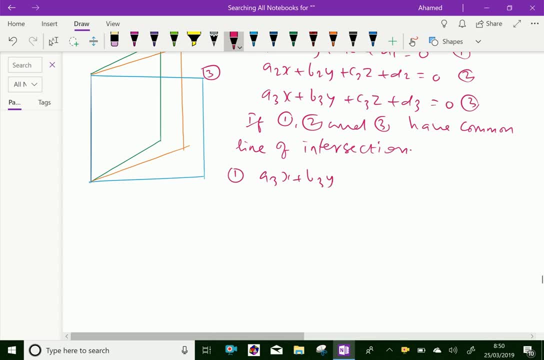 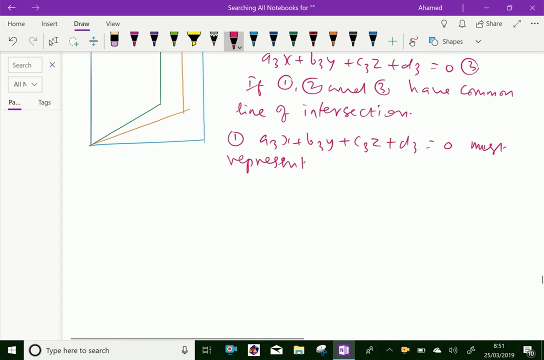 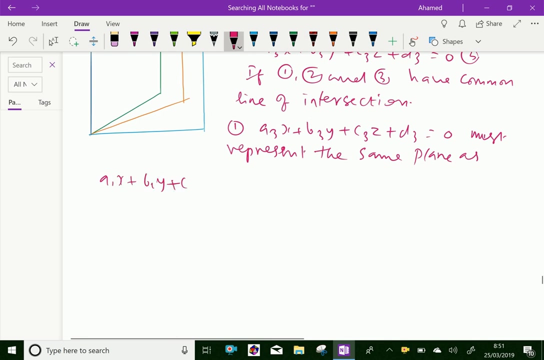 a3x plus b3y plus c3z plus d3, equal to zero, must represent the same plan as must represent the same plan as plan through plan 1 and 2, that is, a1x plus b1y plus c1z plus d1 plus. 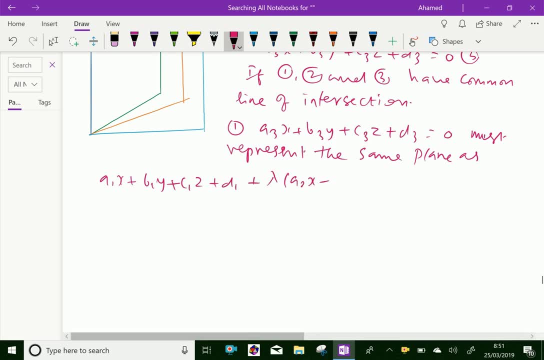 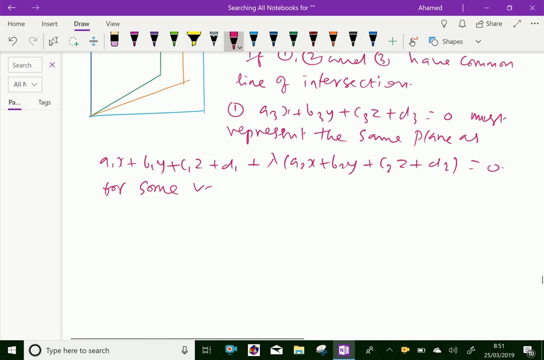 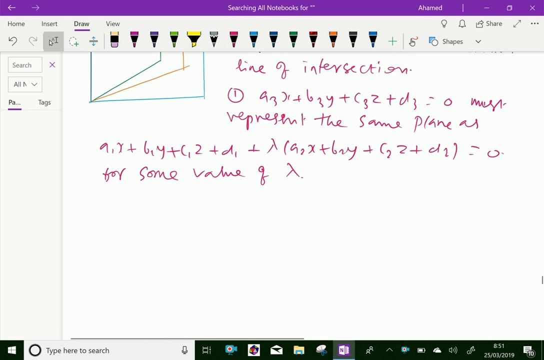 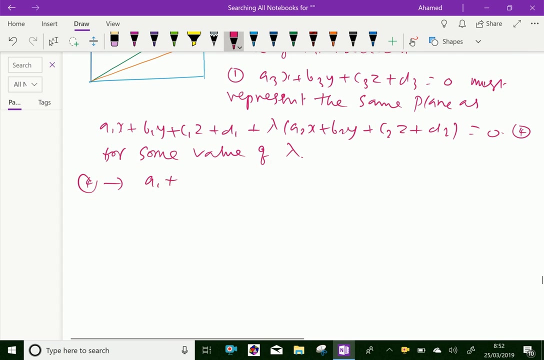 lambda times a2x plus b2y plus c2z plus d2, equal to zero for some value of lambda. for some value of lambda means first: uh, let's keep it. this equation of plan is four. now we can write the four as like: a1 plus lambda, a2x plus a2 plus lambda. 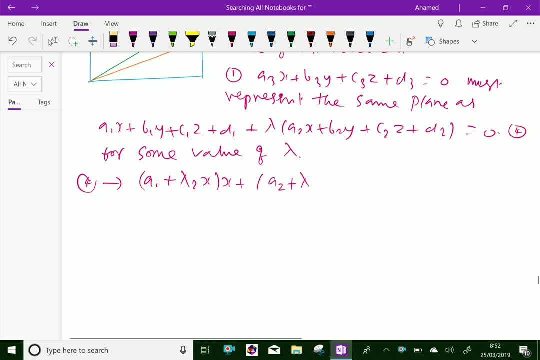 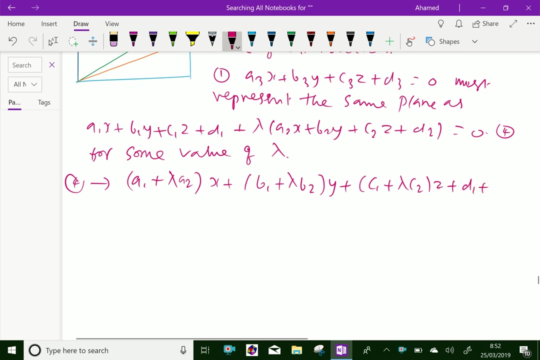 a2 lambda a1 plus lambda a2. x plus a2 a2. lambda chapter, chapter, chapter, them plus b1, b1 plus lambda b2, y plus c1 plus lambda c2, z plus b1 plus lambda b2: equals. 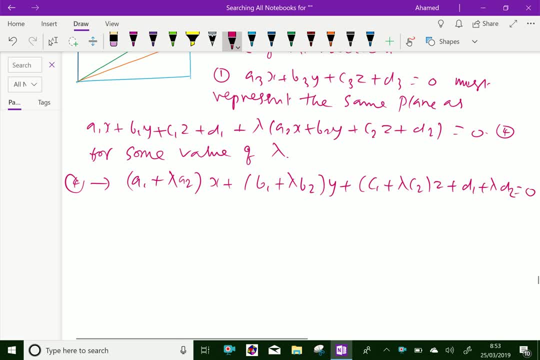 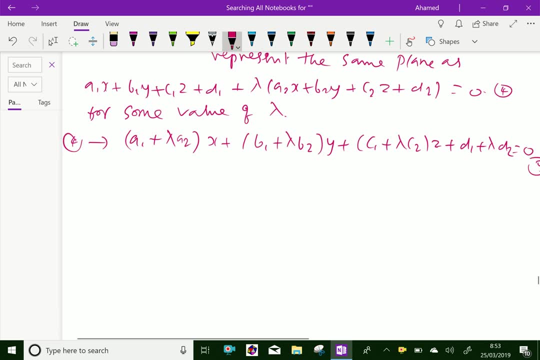 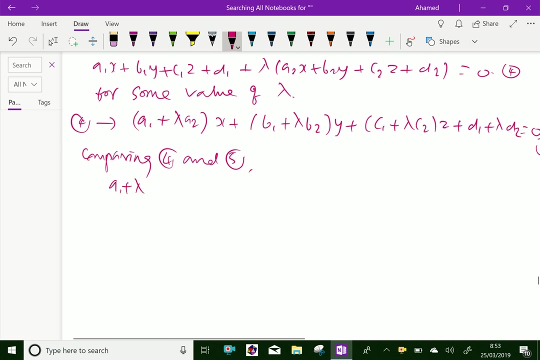 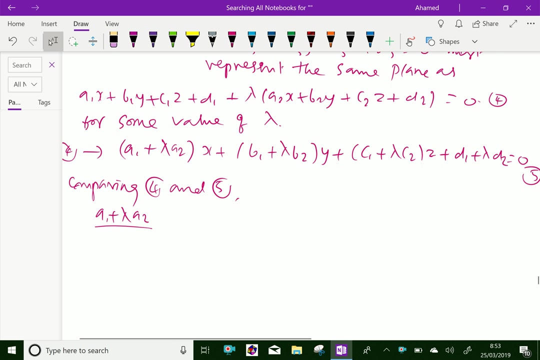 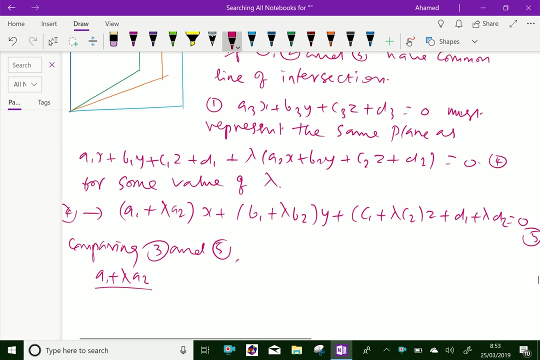 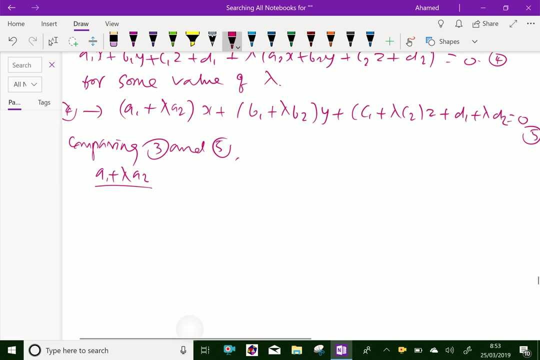 0.. Now let this equation 5.. Now, comparing 4 and 5, 4 and 5, that means coefficient of x is here a1 plus lambda a2, over coefficient of you know, 4 is 3, 3, comparing 3 and 5, coefficient of x in plan 3 is having a 3, equal, like that. 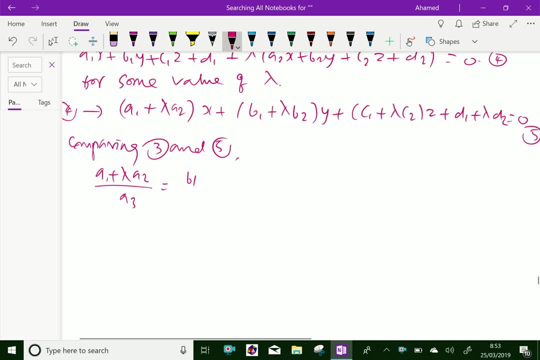 for y coefficient of y is here: b1 plus lambda b2 over b3, like c1, plus lambda c2 over c3, equal b1 plus lambda b2 over b3, all are equal, to let it be k. 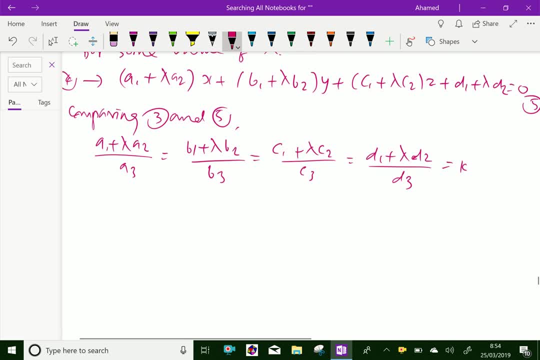 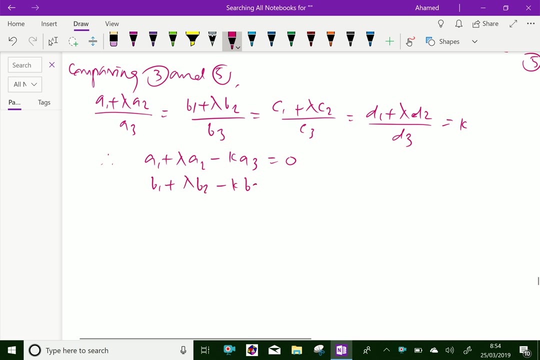 Now therefore, you can see here: a1 plus lambda a2, minus k: a3, equal 0.. Similarly you can write for b: b1 plus lambda b2, minus k: b3, equal. 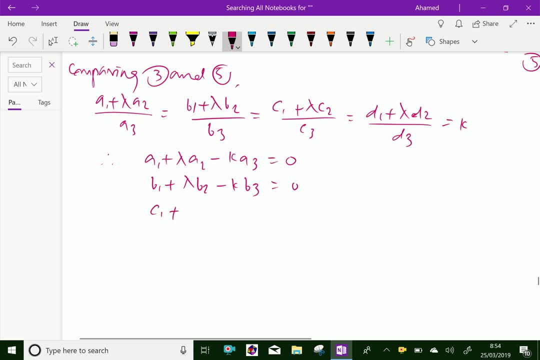 0.. c1 plus lambda c2, minus k c3, equal 0, like b1 plus lambda b2, minus k b3, equal 0.. all let us finish by computing. beta equals lambda b2, minus kd3, equal 0. 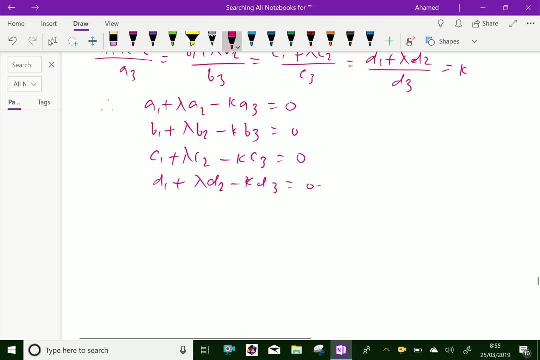 Now this all above 4 equations. let us eliminate lambda and k. by eliminating lambda and k above 4 equations, we are getting determinant. Let it be that 5. Remember, you just need to know impasse values of a point here. if the neutral value of a point there 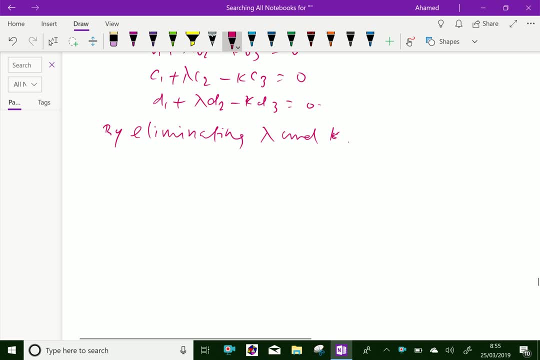 plus the identical value of a point N, you can shuffle back to a nieciane Buchanan. better use Langrange class for oranges. movimento ods. per line 2 to 3.. be that first determinant is Delta, which is equal a1, b1, c1, a2, b2, c2, a3, b3, c3. 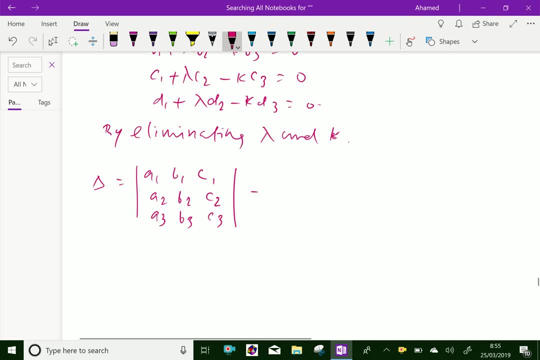 equal 0 and lambda 1 is b1, c1, b1, b2, c2, b2, b3, c3, d3. like lambda 2, equal 0. here, then lambda 2 is a1, c1, b1, a2, c2, d2 and a3, c3, d3. this is for lambda, 2. 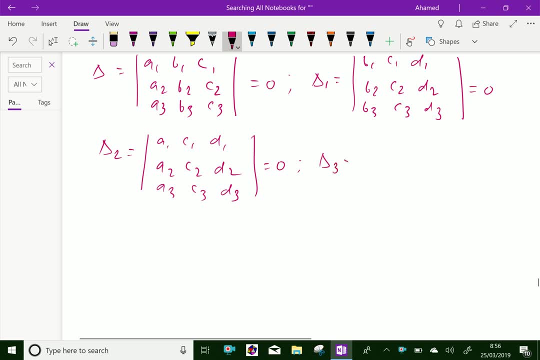 and lambda 3 equal a1, c3, b1, d1, a1, c2, d2, c1, d1. here for lambda 2 is b1, c1. this is lambda 1, lambda 2 is a1, c1, d1 and lambda 3 is a1. 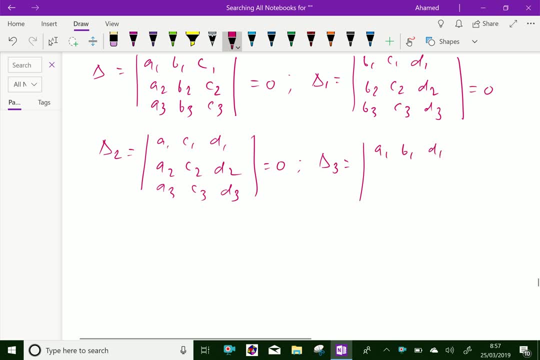 d1, d1, that is, c1, c2, c3 are eliminated here, like a2, b2, d2 and a3, d3, d3 equal 0. these are which are the required condition. if here you can get a condition for if, if the plan, if the plan above three plans intersect. 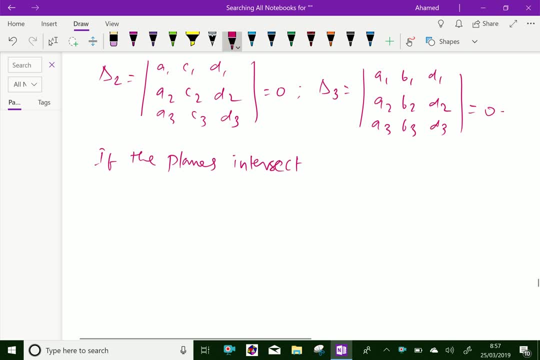 intersect in your line, in your line, then then delta, that means delta, comma delta 1, delta 2 and comma delta 3. all are equal to zero, all, all should vanish, meaning, meaning all determinant value is zero. then we can say: these plants intersect in a line. 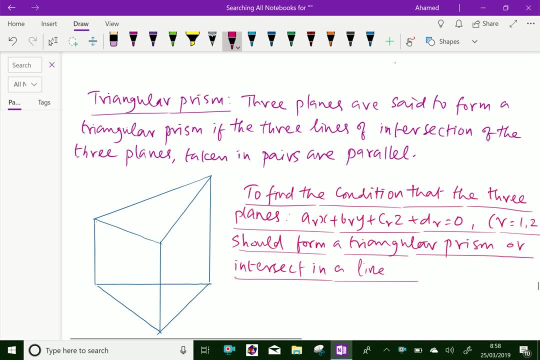 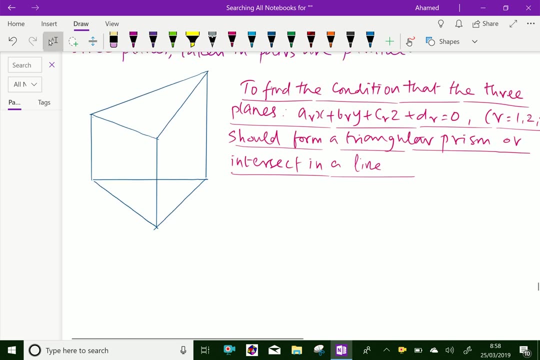 now let us do some other conditions like: uh, how to form a triangular prism? three plants set to form a triangular prism if the three lines of intersection of the three plants taken in pairs are parallel. here suppose this is a plan one, this is a plan two and this is a plan three means all vertical here. 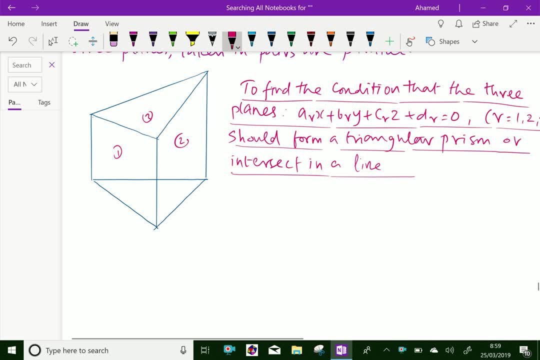 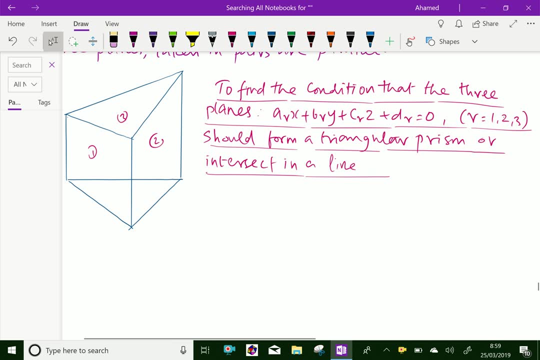 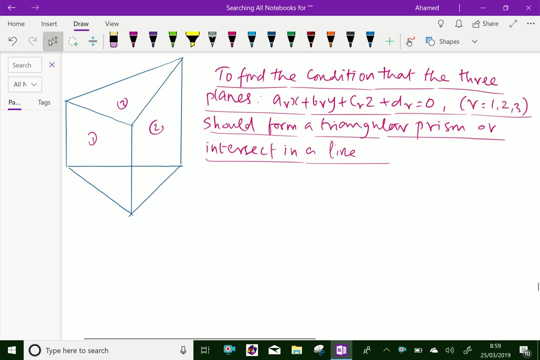 to find the condition that three plants, that is arx plus bry plus crz plus dr, equal zero, that is r equal to one, two, three, should form a triangular prism or intersect in a line. here already we discussed about these three plans and its determinants. we found then, if 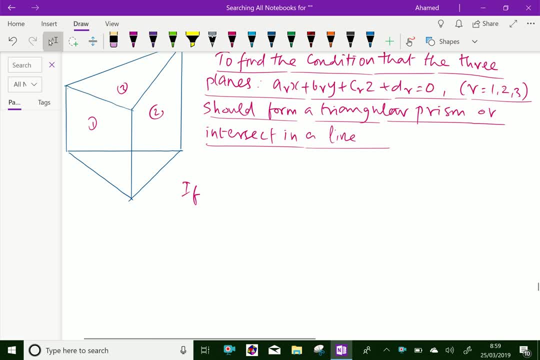 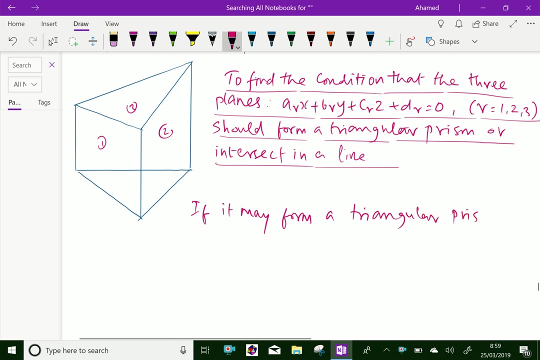 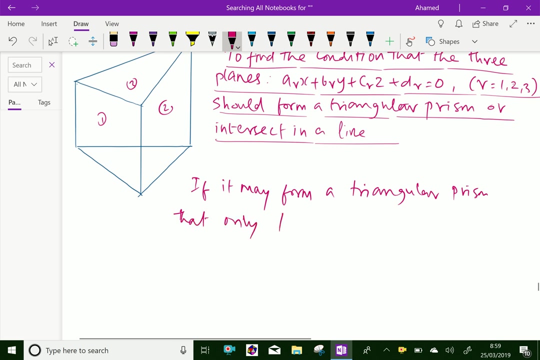 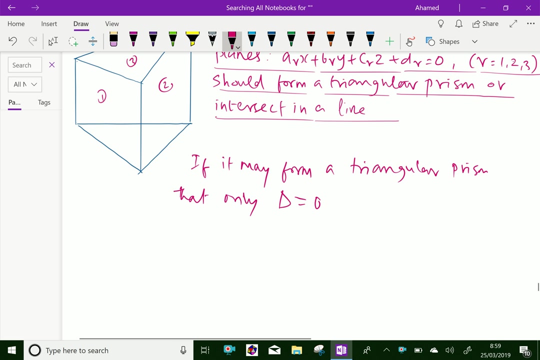 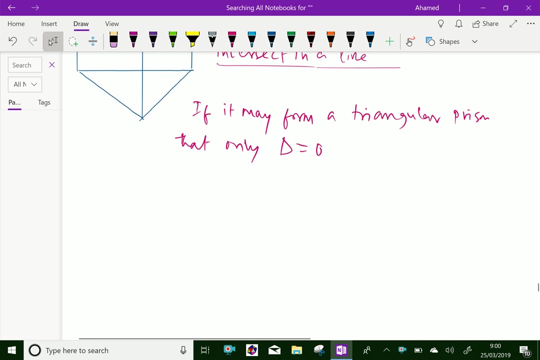 if, if it may, if it may form a triangular prism. triangular prism that that only delta equal zero means, if only delta equals zero, not other determinants, then we can say: these three plans form a triangular prism. now, other condition: they may intersect. this, that means, the three plans they may intersect. 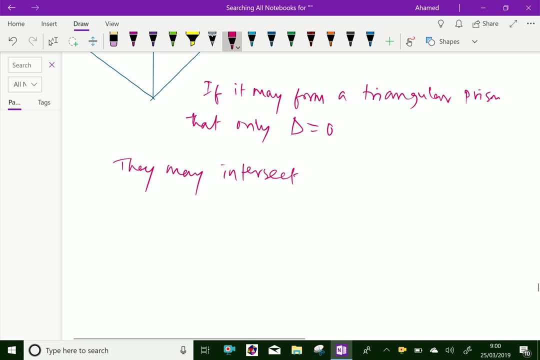 they may intersect in a unique finite point in here unique finite point means all intersect between one point, then it should be equal. then we can say delta should not be equal to zero. this is the condition for these three planes intersect in one point here collectively. we will see now if 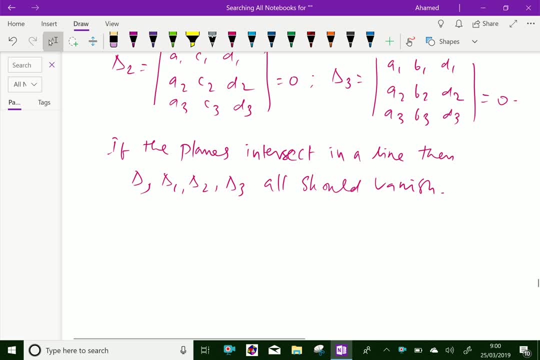 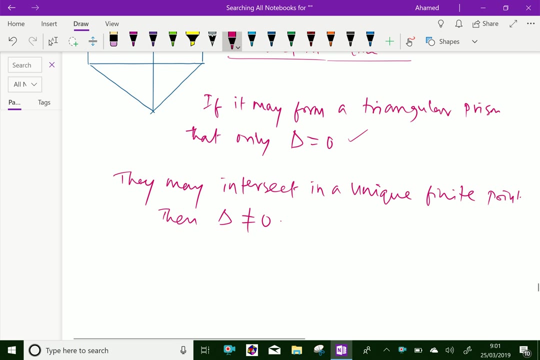 if delta delta one, delta two, delta three, all should vanish. that means all are equal to zero. then we can say these three plans intersect in lines, then if may form a triangular prism, that only if delta equal to zero and they may intersect in a unique finite point, then delta equal delta, not equal to zero. 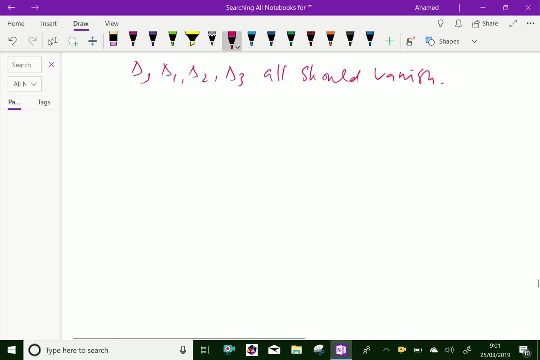 we have done. please subscribe our youtube channel. please subscribe our youtube channel.